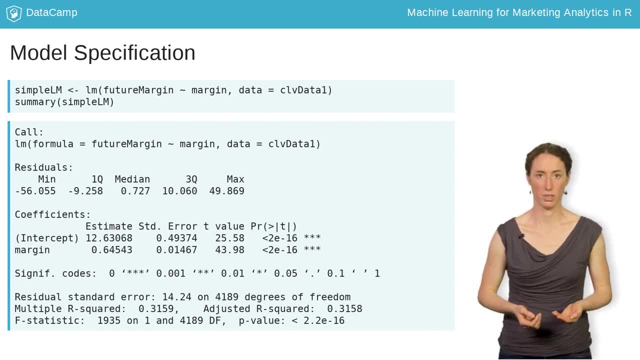 in year 1,, the higher we expect the future margin to be. Also take a look at the multiple R squared at the bottom of the output. A value of roughly 0.32 means that about 30% of the variation in the future margin can. 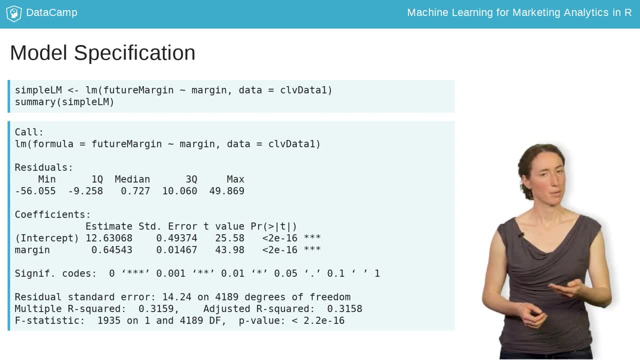 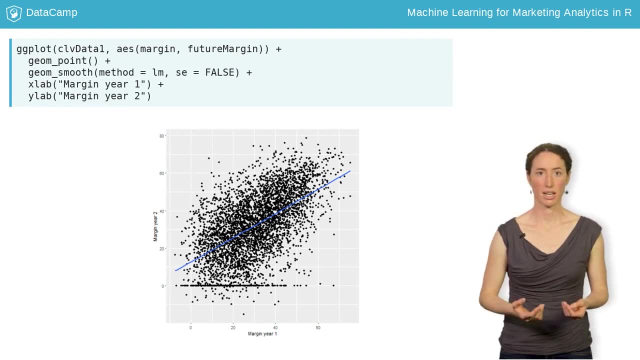 be explained by the margin in year 1.. But more on that later. The ggplot function from the ggplot2 package gives us a nice visualization of the relationship. Here we produce a simple scatter plot of the observations using our clvdata1 dataset. 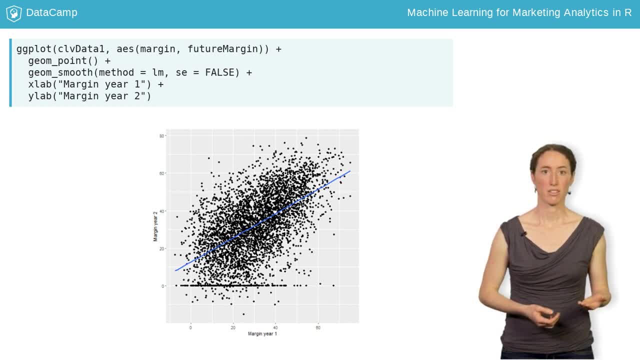 The data is the first argument And we specify margin as the x-axis and future margin as the y-axis in the AES call. This is the second argument to ggplot. We also use geom smooth with method equals lm to fit a linear regression line through. 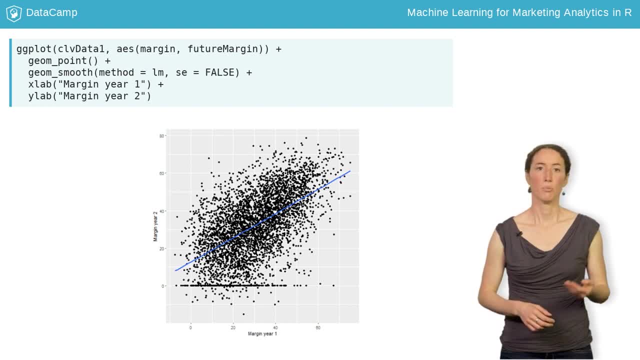 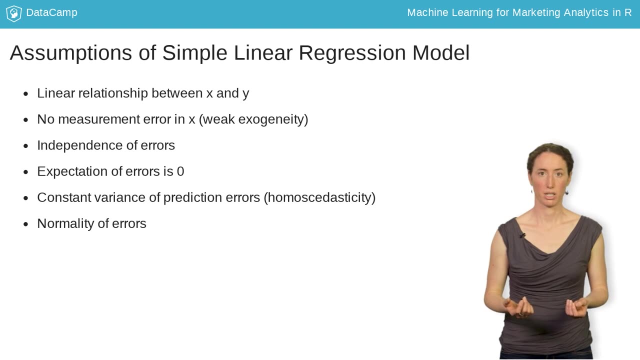 the data cloud. Before moving on to multiple linear regression, let's take a look at the conditions that the data must satisfy for linear regression to be the best method. The relationship between the independent variable and the dependent variable should be linear. The independent variable should not contain any measurement errors. 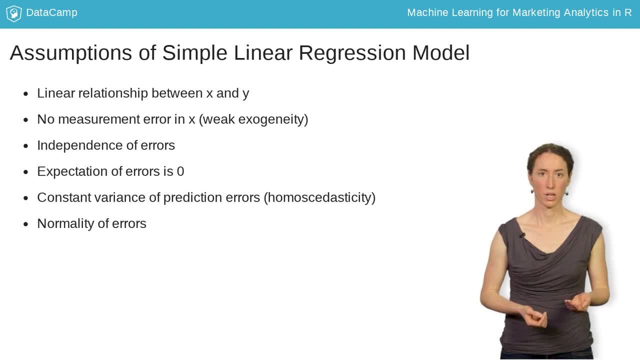 The residuals should be uncorrelated. One cause of correlation among the errors is violation of the linearity assumption. The residuals should randomly vary around zero and their expectation should be equal to zero. Usually this assumption is not problematic as long as a constant is included in the model. 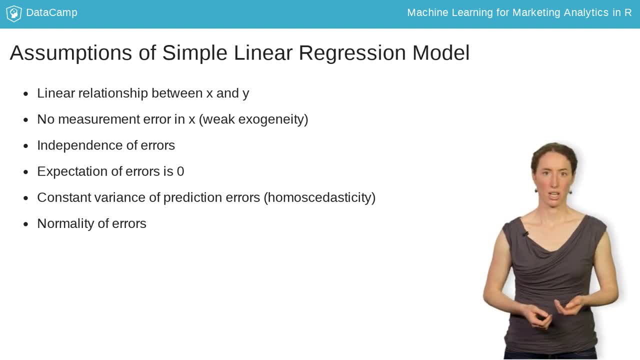 The result is a linear regression. The variance of the prediction error has to be constant. If not, inferences made from the model can be misleading. When doing statistical significance testing, we also have to assume that the errors are normally distributed. A well-established method to check the violation of these assumptions is a plot of the predicted. 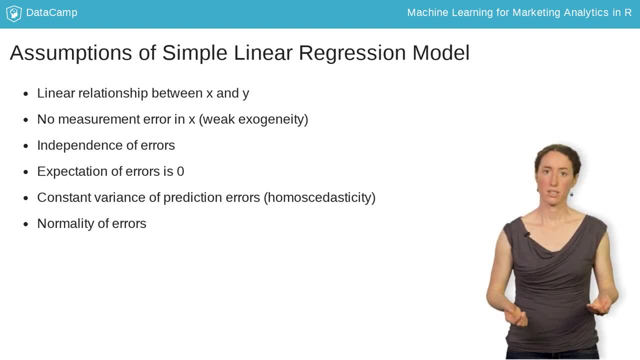 values against the estimated residuals. This is called a residual. Now let's try some examples.